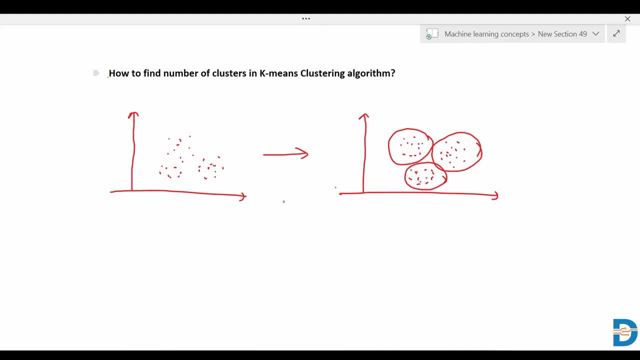 in k-means clustering. how many clusters the algorithm should take. Okay, So clusters can be: k equals to one, k equals to two, k equals to three, and many more. So how to decide that, how many clusters it should consider, It is decided with the help of Albo. 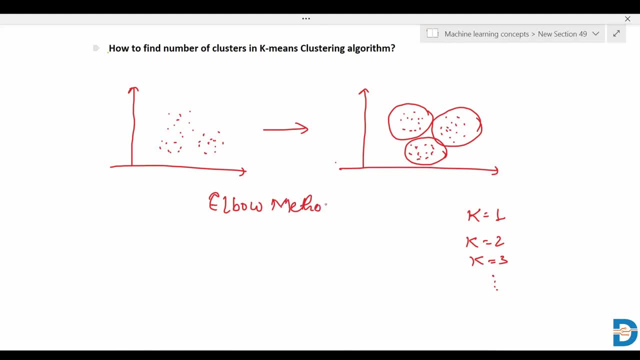 method. Albo method is used to decide how many clusters it should take. So how many clusters it should take, It is decided with the help of Albo method. Okay So, what is Albo method? So Albo method is basically graph between k and WCSS. Okay So, 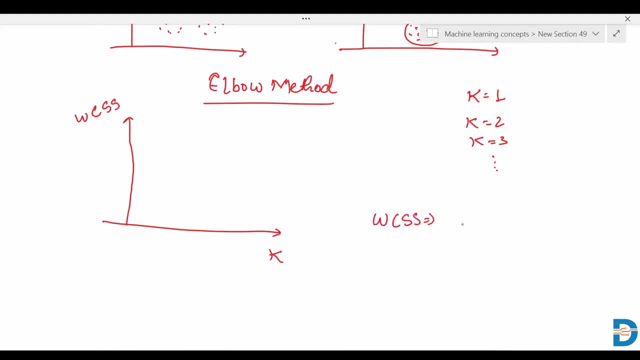 what is WCSS? first, WCSS is the sum of squared distance, sum of squared distance between, between, between each point and the centroid of the cluster, of cluster. So it is within cluster, sum of squares, within clusters, sum of squared. Okay, So this is, this is WCSS. So what basically we do in Albo method? 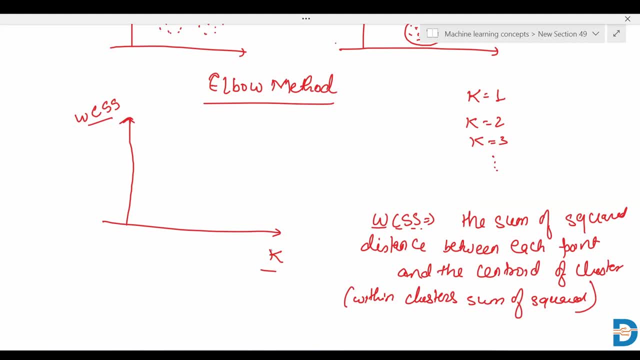 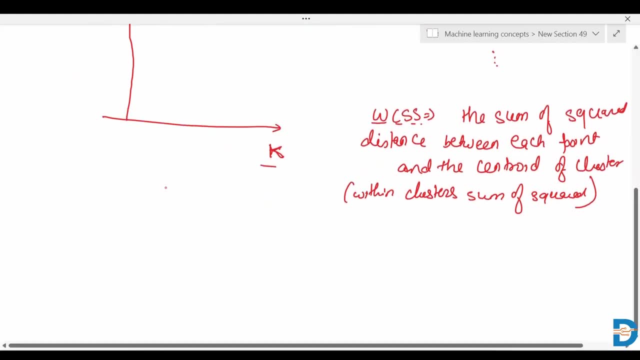 We will make graph between WCSS and k. For each value of k, we will calculate WCSS and we will make the graph. Okay, So let us understand that how to calculate WCSS. Okay, So, for example, we have: 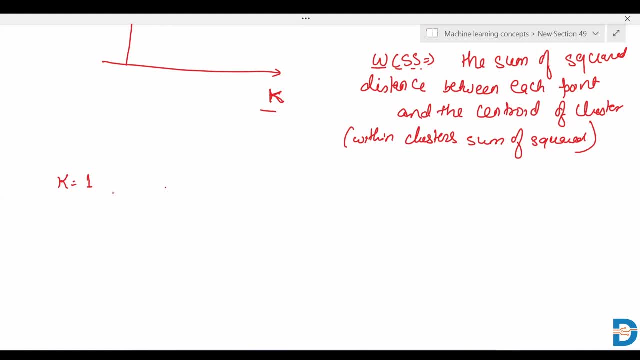 we have taken k equals to one. that is only a single cluster. Okay, So all the data points will belong to a single cluster. Okay So, for example, this is centroid of that cluster and these are the data points. Okay, So, from the cluster, from each data point, it will find the 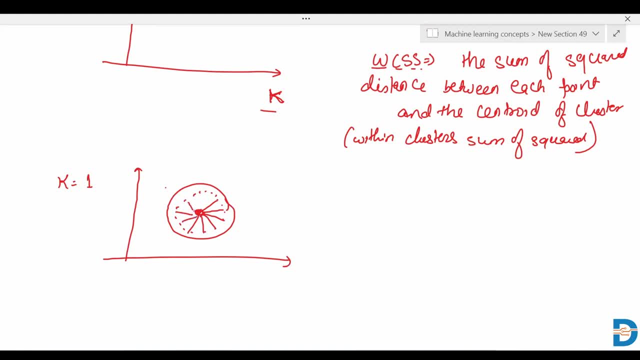 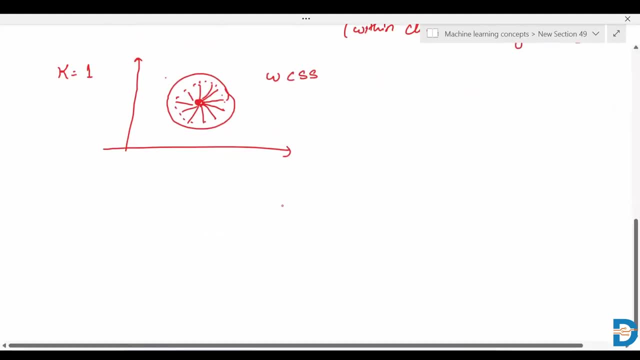 distance and square it. Okay, So sum of these is known as WCSS. Okay, Now let us consider that we are considering. k equals to two means, two number of clusters. Okay, So the all the data points are grouped into two clusters. 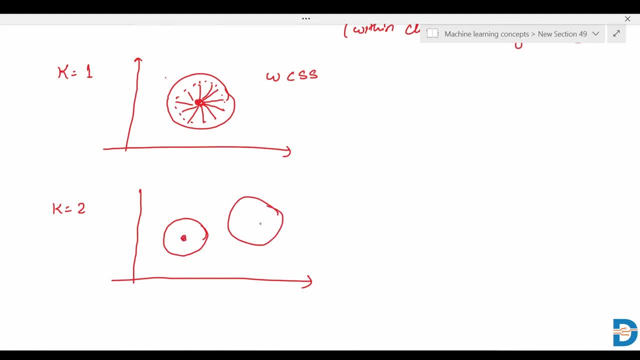 So two clusters have this is centroid for this cluster and this is centroid for this cluster. So we have data points here and data points here. Okay, So it will take distance from each of the data points and centroid, Okay, For this cluster. also, it will take each distance from centroid to. 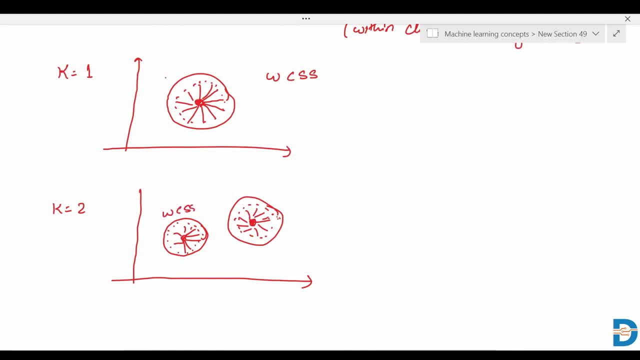 each data point. So this is WCSS for cluster one and WCSS for cluster two. So total WCSS will be WCSS1 plus WCSS2.. Okay, Again, we are considering that k is equals to three. So the data points are grouped into three clusters. Okay, So this is. 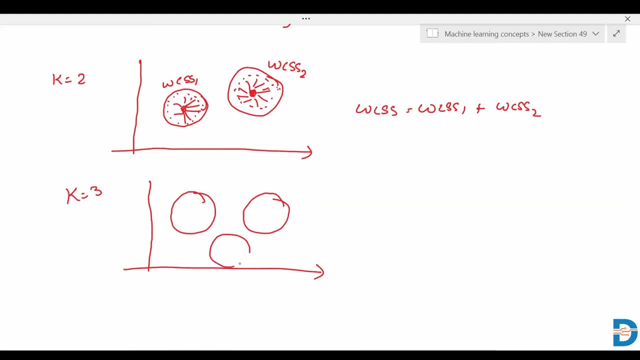 cluster number one, cluster number two and cluster number three. Every cluster has its own centroid, So the data points belonging to this cluster, these data points belongs to this cluster, these data points belongs to this cluster. So again it will find the 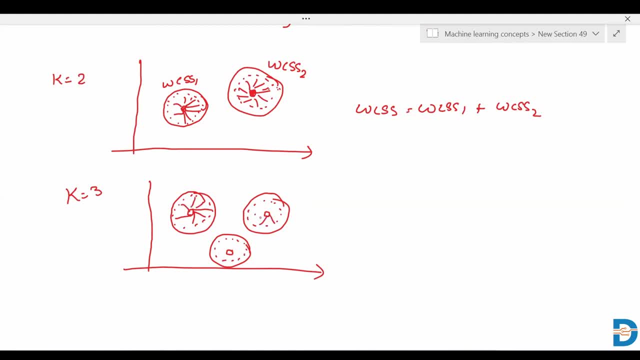 distance between centroid and data points. for this cluster also, and for this cluster also. So, for example, this is the distance: WCSS1.. For this cluster it is WCSS2 and for this cluster it is WCSS3.. Okay, So total WCSS is equals to WCSS1 plus WCSS2.. 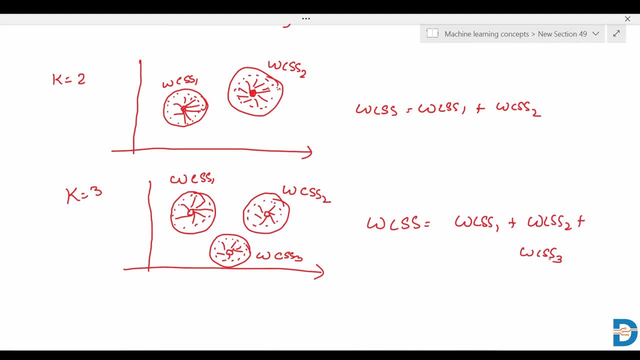 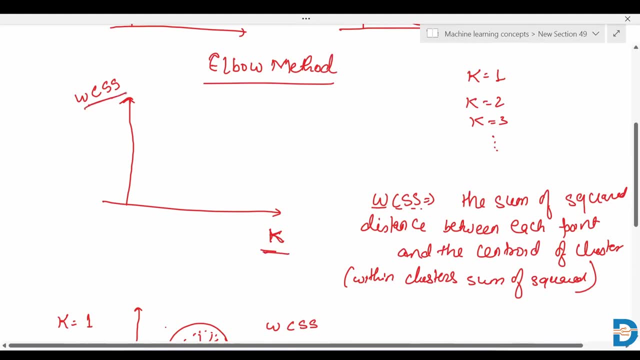 Plus WCSS3.. Okay, So we will make according to number of, we will increase the value of k and we will find the WCSS. Okay, So, when we will do that, we will obtain a graph like this: So this is in the shape of elbow. Okay, So this is for: k equals to 1,. k equals to 2,. 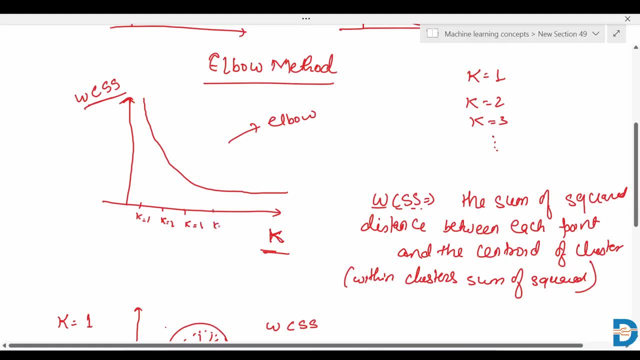 k equals to 3, like that, And it is k equals to 2.. So this is for: k equals to 1, k equals to 2, k equals to 4, like that. It will increase. So where this elbow will come, where this elbow. 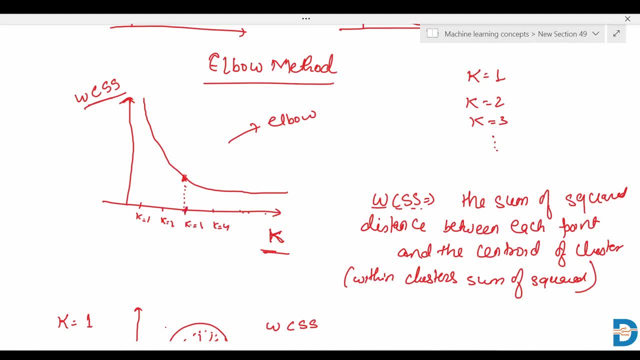 will come, we will consider that number of clusters. So for example, here we can see that elbow is there at k equals to 3.. So for this particular curve we will consider that we will group the data points into three number of clusters. So this is the way we will decide.